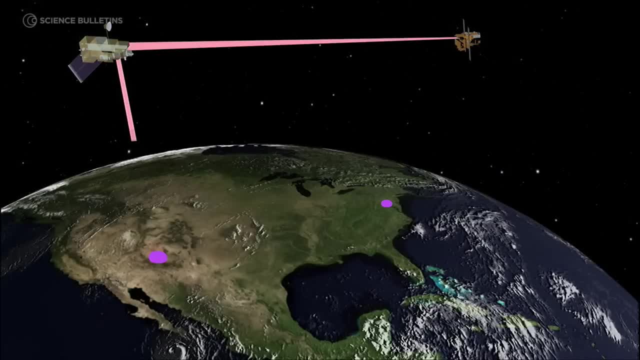 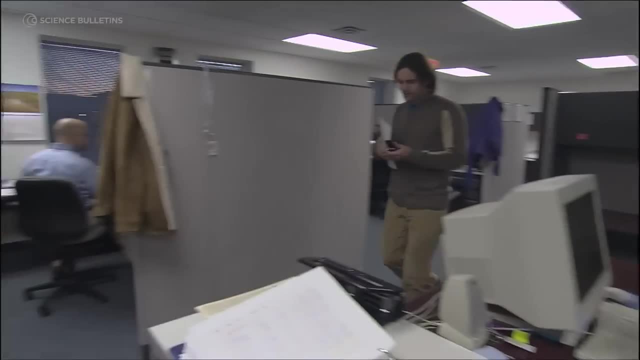 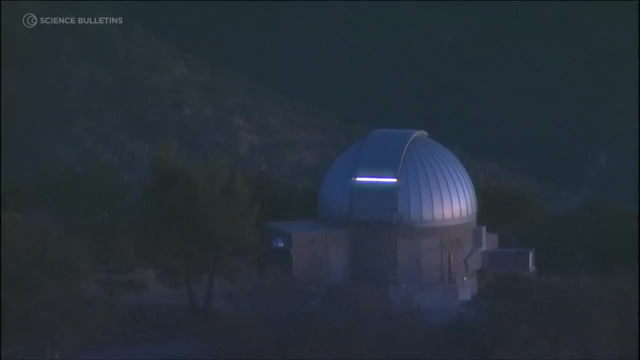 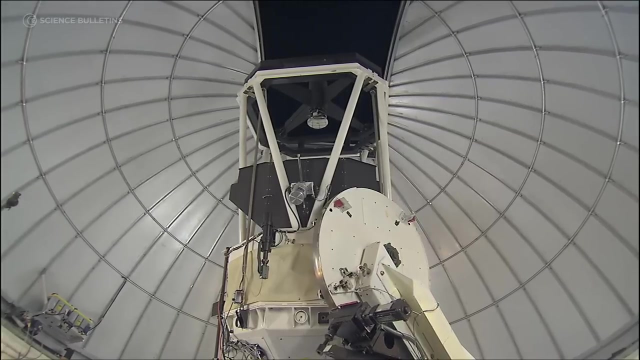 The data from the burst immediately flow down to the ground and they're distributed on the Internet. That allows ground-based telescopes to point at the direction of the burst quickly. What we've known now for a decade is that when a gamma ray burst goes off, 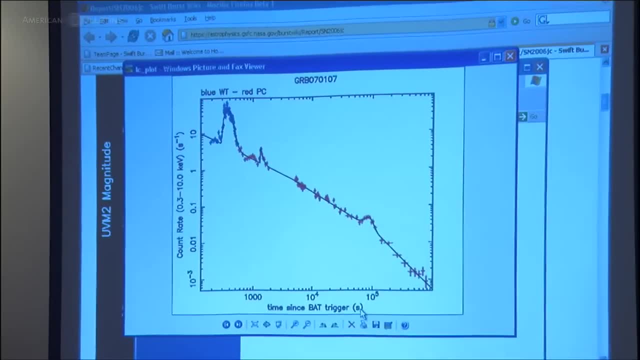 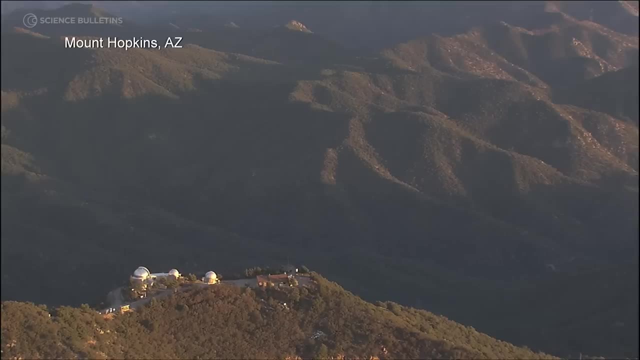 it leaves behind this dying ember, this afterglow light, And we can use the traditional telescopes, those that are sensitive at optical and infrared wavelengths, to be able to study the details of how the light's changing, how the colors of that light is changing. 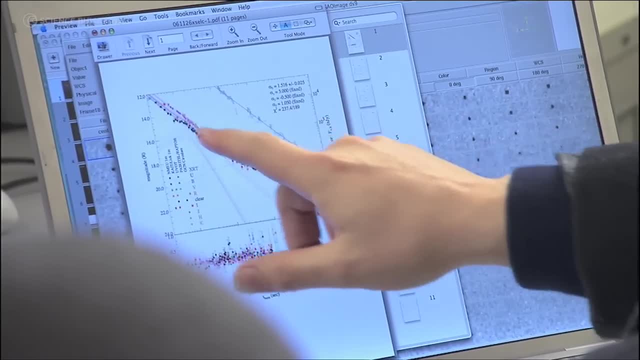 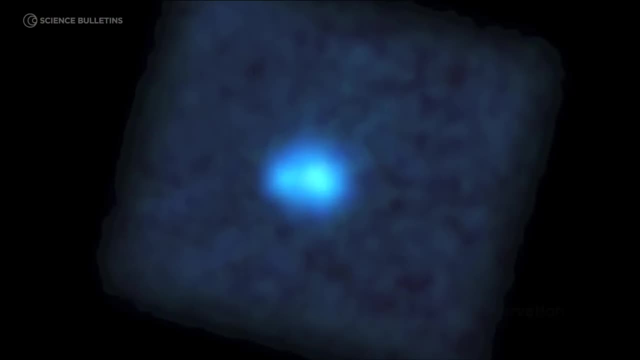 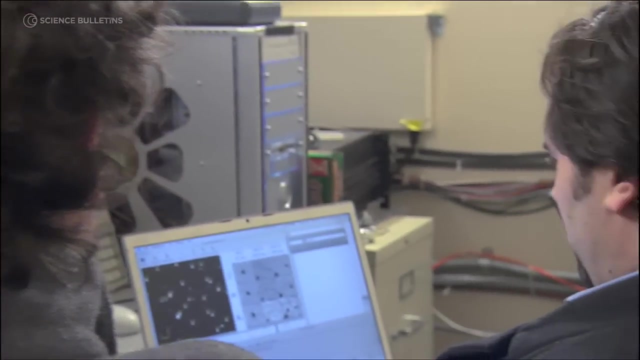 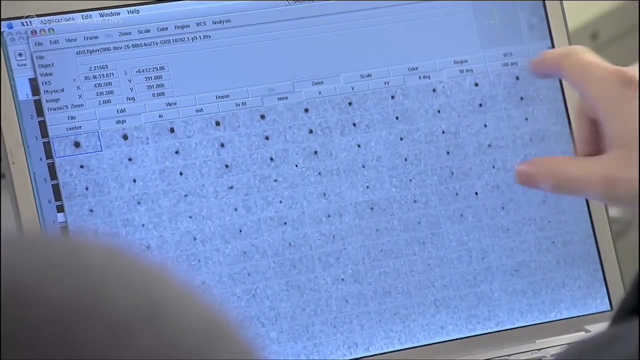 And in those details we can uncover some of the physics of the explosions. This is the afterglow, 58 seconds after the gamma ray burst triggered the Swift satellite, And you can see that it's fading from black all the way down to nothing. 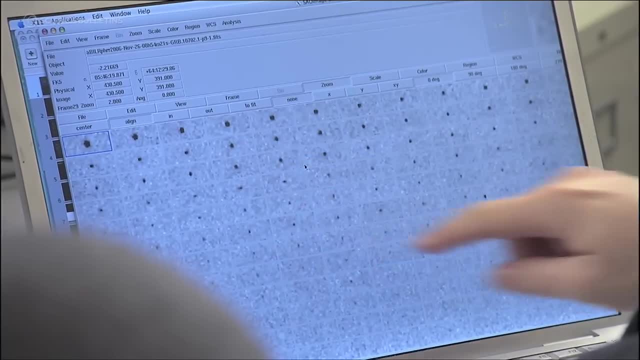 We start off 58 seconds and then 30 minutes later we really don't see anything. It fades really fast. Oh yeah, it fades very quickly. It's a good thing that we got on so early. Yeah, quick response. 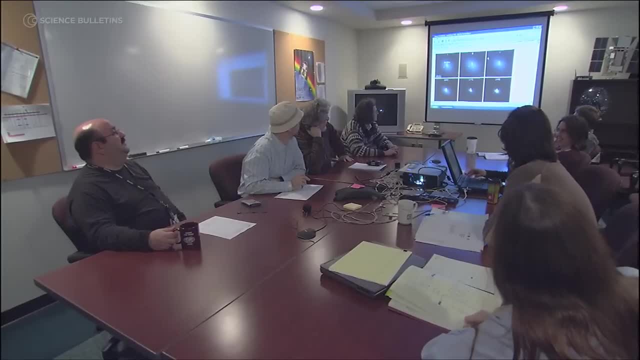 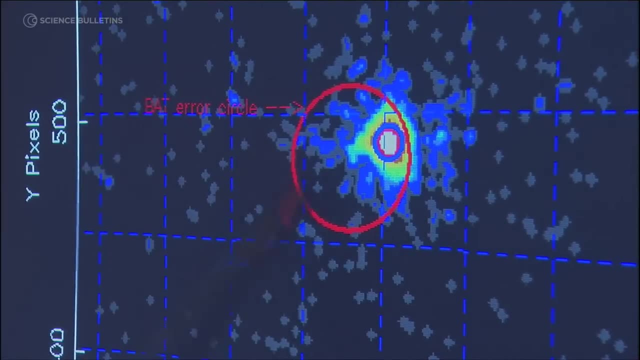 When you look at each gamma ray burst in detail, you see very, very different things, And it's turning out that, as we're learning more about gamma ray bursts, we believe that those differences actually amount to differences in what makes the gamma ray bursts. 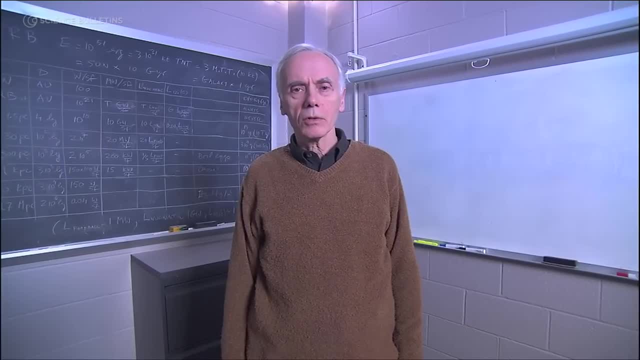 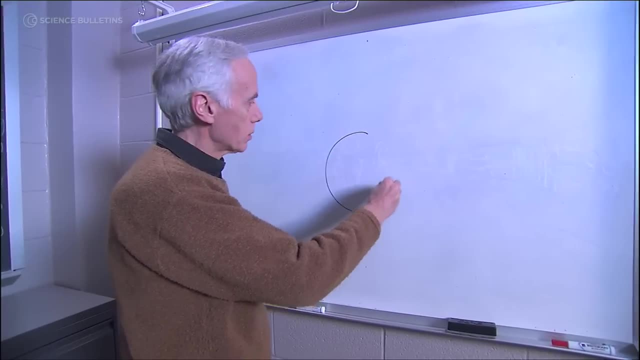 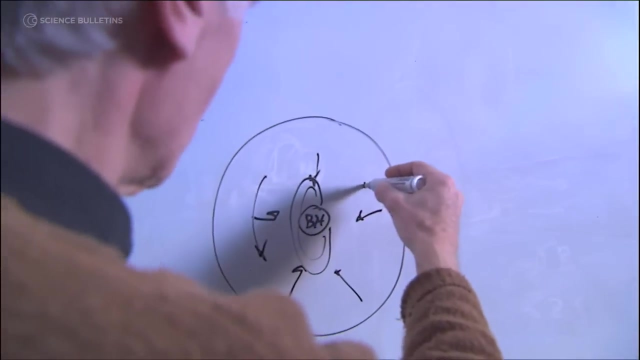 Based on observations and what we know from physics, there are two types of models that have come to be representative of gamma ray bursts. We think that they originate in a massive star which collapses to a black hole. The star is rotating so that the material that falls in forms an accretion disk. 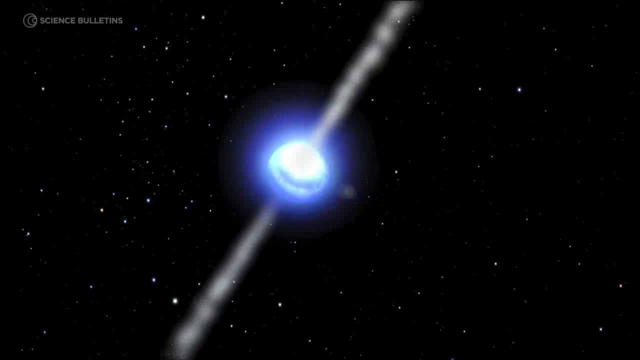 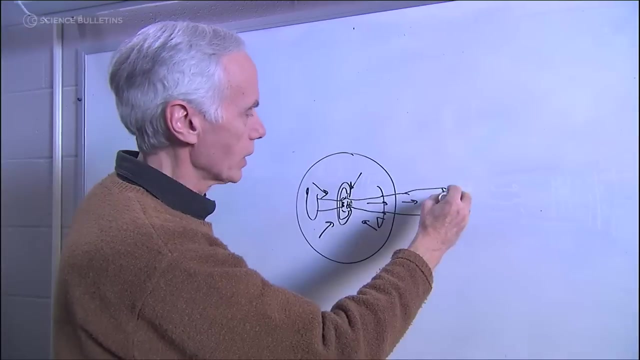 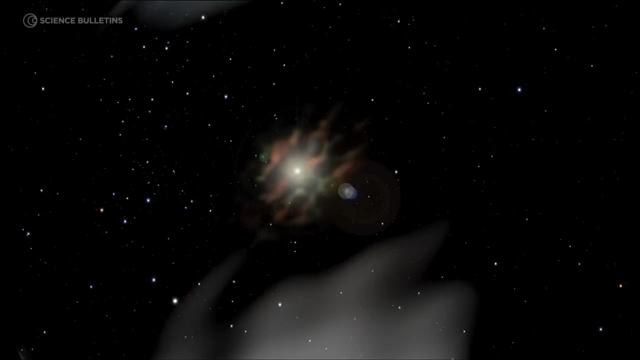 And that produces a lot of energy, which creates a relativistic fireball, resulting in a jet being ejected along the rotation axis, Creating gamma rays, And those gamma rays are thought to give rise to the gamma ray burst. There is a second model.